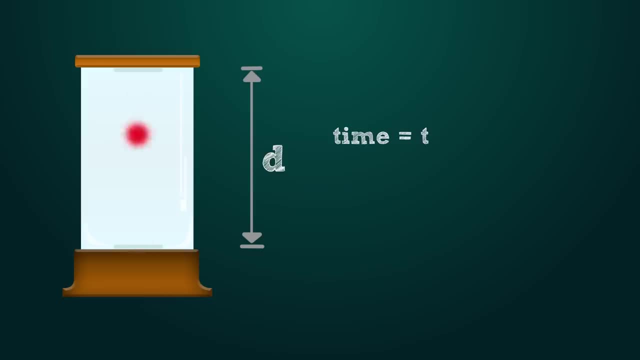 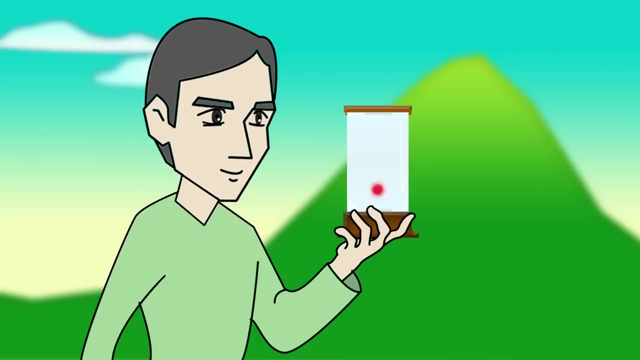 and the time for the light to cover that distance is t. For the sake of simplicity let's say it's one second. So when this clock is with you at rest position, the light bounces between the mirrors, covering distance d in one second. 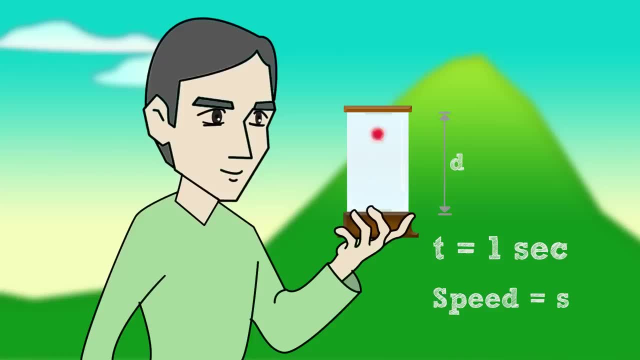 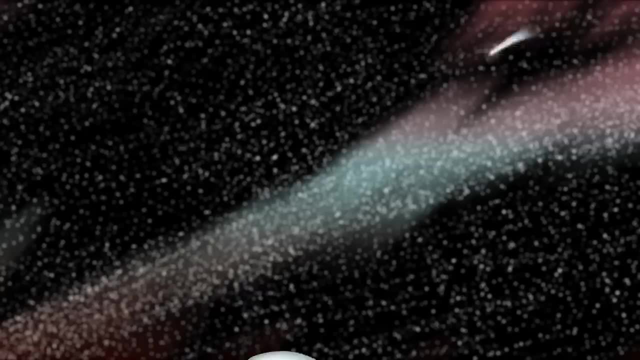 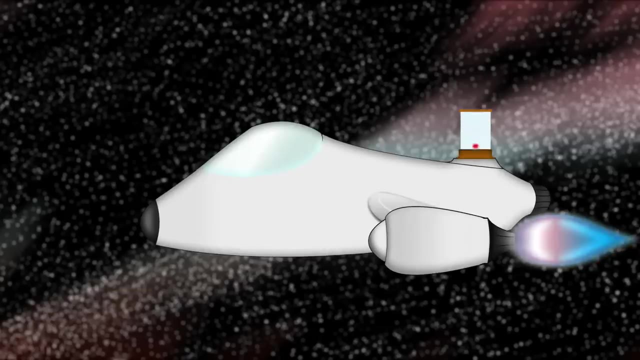 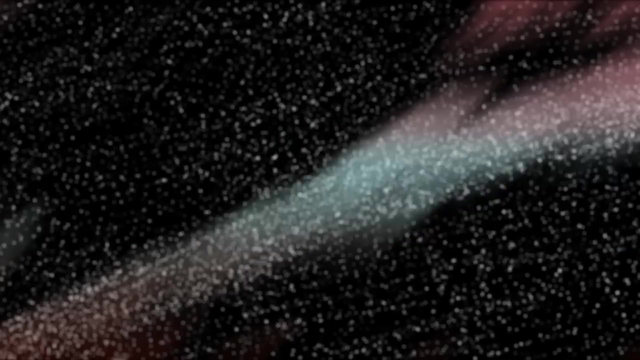 which gives us the speed of light s. Now remember: speed is distance per unit time. Now consider: Einstein also possesses the same light clock with him, Only this time he is travelling in a spaceship along with the clock. When Einstein travels in a certain speed, 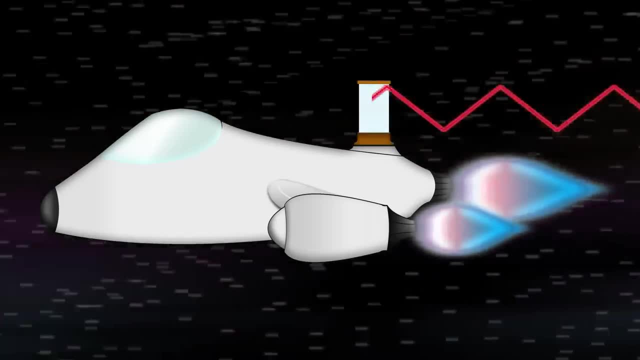 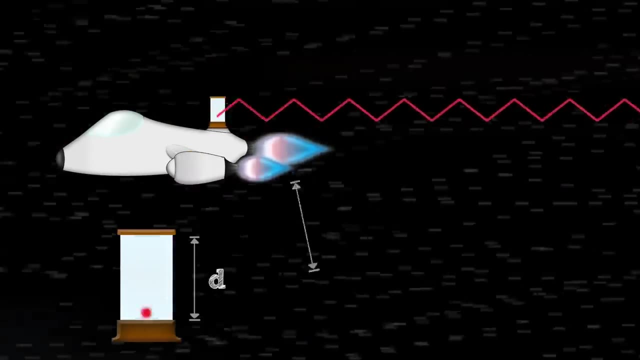 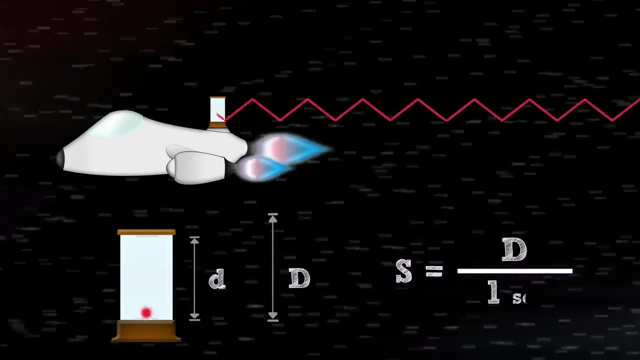 the clock travels with the clock, With the same speed of the spaceship, in the same direction. Here light has to travel an extra distance in the same one second. Let's consider this distance to be capital D and represent the speed of light here as capital S. 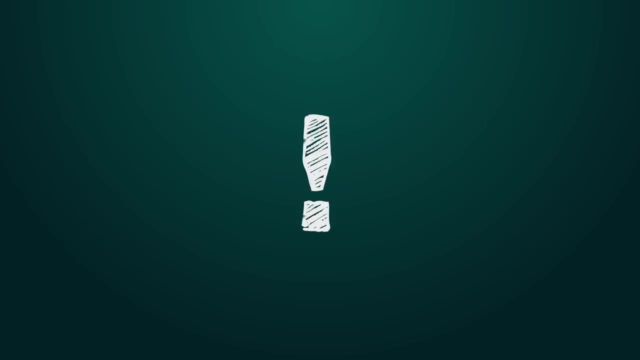 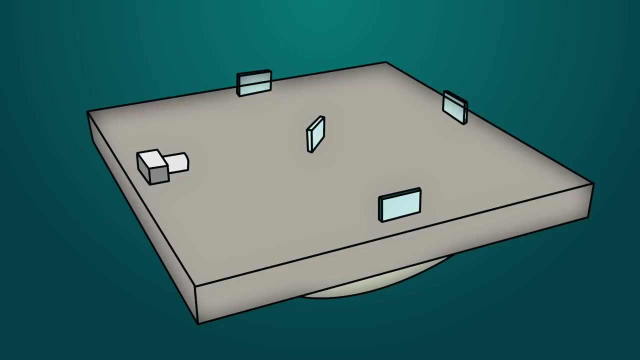 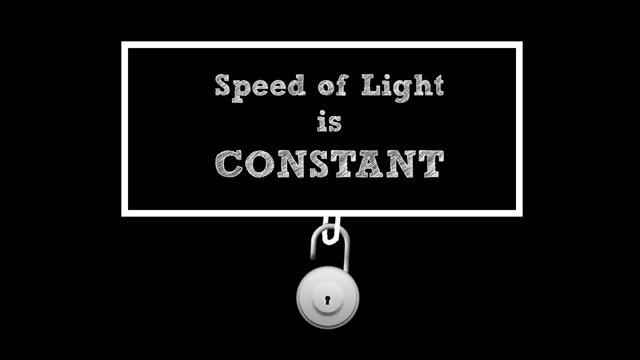 which has to be greater than small s. But something's wrong here, Because in the late 1800s the Michelson-Molly experiment tried to detect the relative motion of the matter through an ether And concluded that the speed of light is constant. 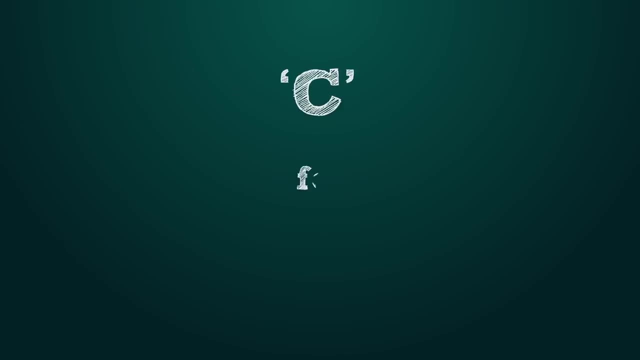 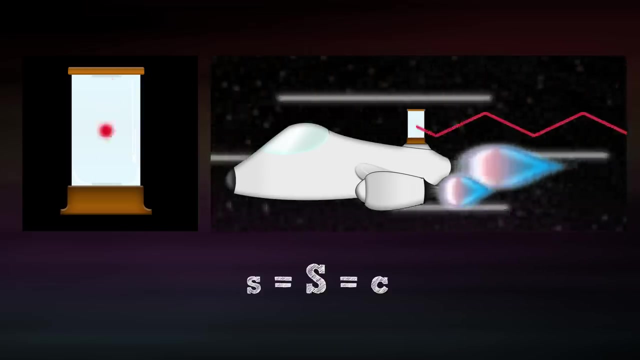 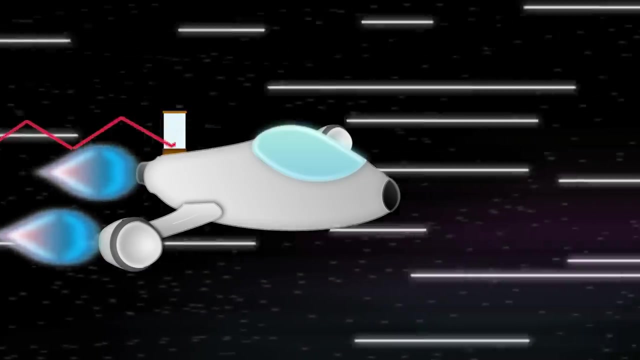 This cosmic speed limit is known as c, So in our little scenario, small s and capital S are equal. So for the speed of light for both you and Einstein to remain constant, something has to give way, That something is time. 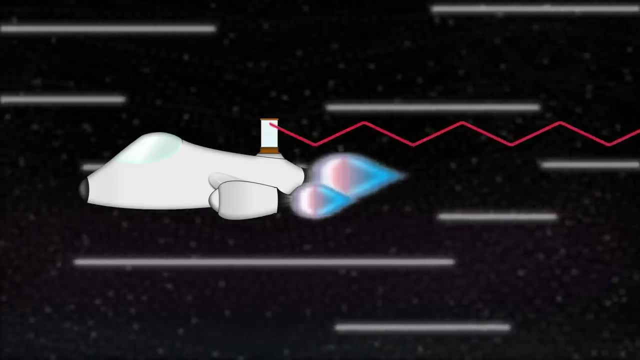 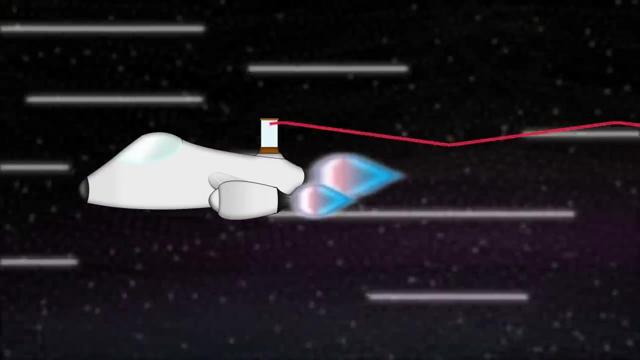 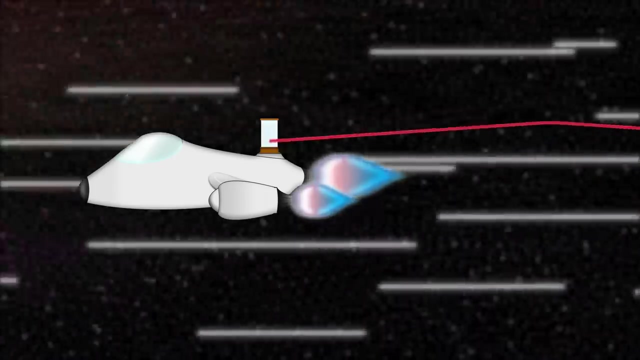 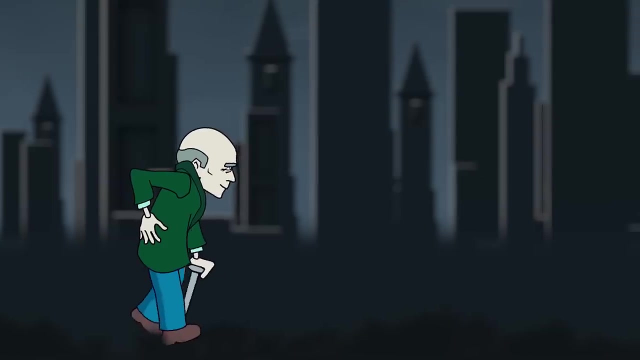 It turns out, time slows down when you travel faster and faster, nearing the speed of light. So the faster Einstein travels, slower the time passes for him. Hence, what could be a day for Einstein in space could be as much as 50 years for you on the ground. 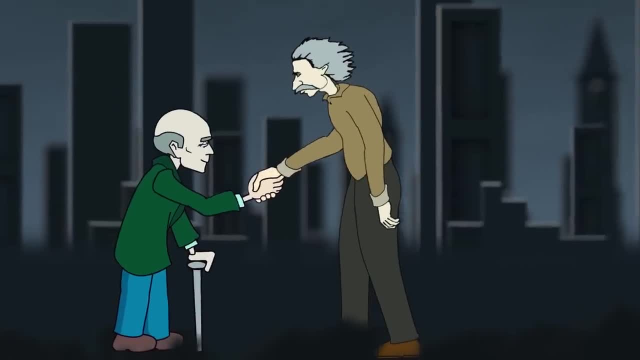 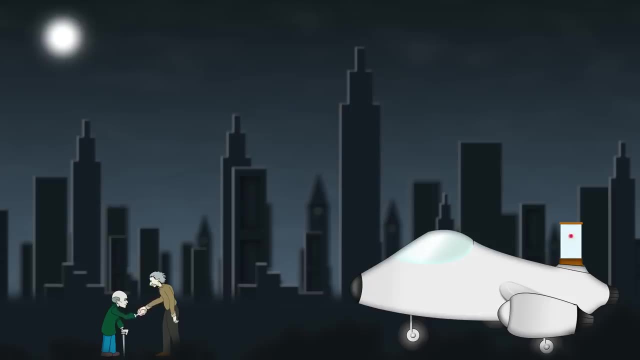 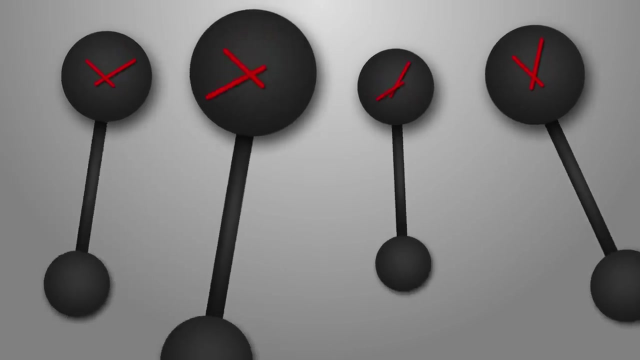 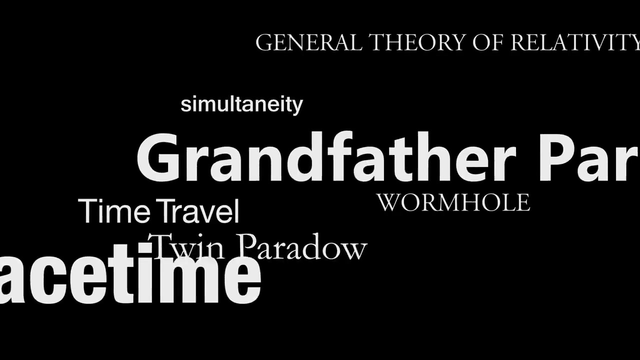 This became the fundamental conclusion of the theory of relativity, a theory proposed by Albert Einstein in 1905.. This theory broke the traditional understanding of time as a constant entity and proved that time, in fact, is different for different observers. The theory of relativity led to many other invaluable findings.